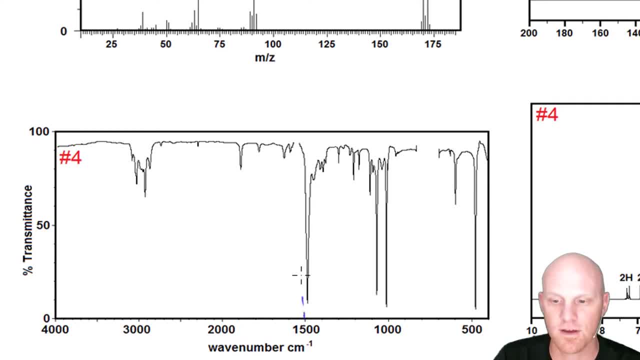 spectrum. if we look, we want to just kind of look at everything outside the fingerprint region, So kind of map out and everything left of 1500 and technically it's really a little less than 100.. So it turns out this peak right here will end up being significant. but 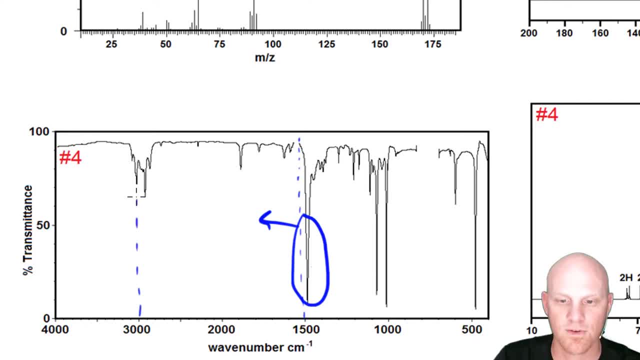 here's 3000.. If we just kind of mark up where 3000 falls, there's 3000 working its way up and we've got peaks both on the right and on the left of 3000.. The ones that are immediately to the left are the sp2 CH bonds and the ones that 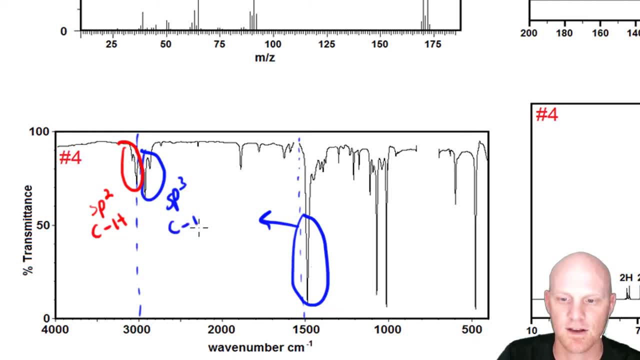 are immediately to the right are the sp3 CH bonds. So having these sp2 CH bonds, that's either usually part of an alkene or an aromatic ring. We don't have a signal of any significant strength around 1650, so I don't think alkene, but we do have again this signal right here. So and 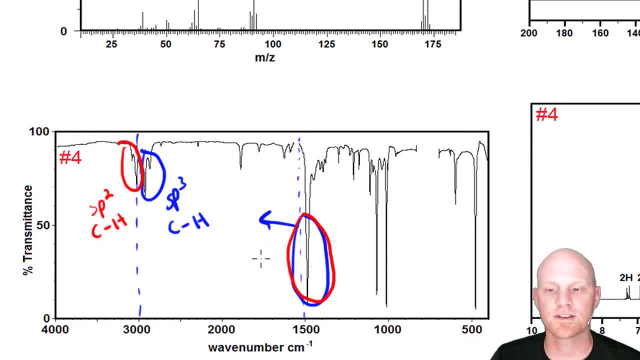 again, from a little less than 15, technically, to a little more than 1600. you might have one, two or three peaks and that's your evidence of a benzene ring, So an aromatic compound. and in this case, even if we weren't completely positive with a benzene ring here, the NMRs will definitely clue us in. So let's. 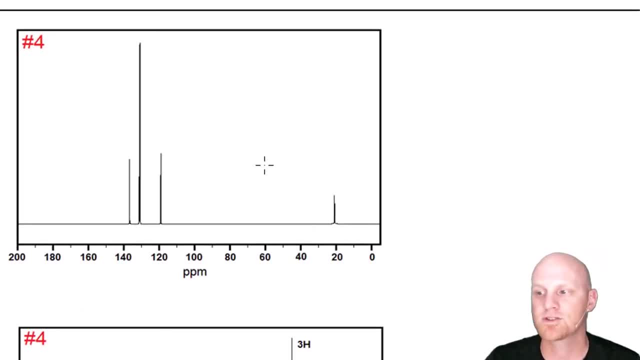 take a look at that carbon 13 spectrum. now We're not going to spend too much time here either, but we've got four signals. So we've got an alkane signal down here, and then these are all in the 110 to 160 range and most likely 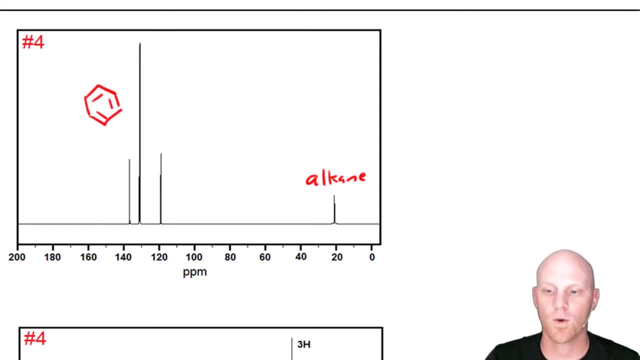 aromatic signals, So confirming what we kind of speculated over here on the IR, that that peak was indeed an aromatic carbon, carbon peak In this case. I'm going to be a little nice for a second. if I was given this to some students in a laboratory setting I probably wouldn't say a thing, but on an exam most. 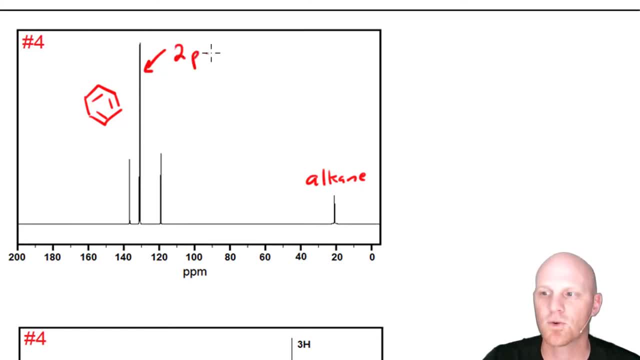 professors would be nice enough to kind of point towards there and say that's actually two peaks. So it looks like from the NMRs we've got a little bit of an initial inspection that there's really five signals in this thing. but I'm telling you that this thicker peak in the middle here is actually two peaks all. 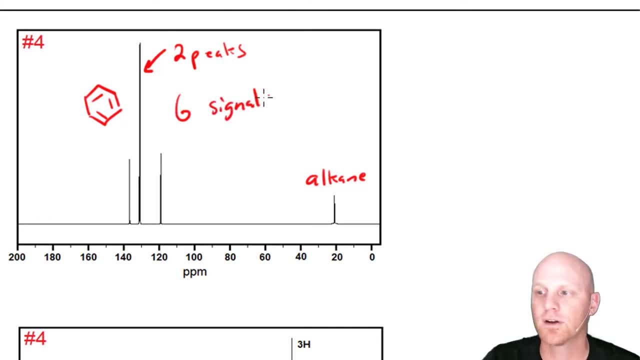 on its own, and so there's really six signals here. so in the HNMR, and so four signals in the aromatic region, tells me that we've got some symmetry in our benzene. Benzene's got six carbons, so it'll only have four signals. there's some. 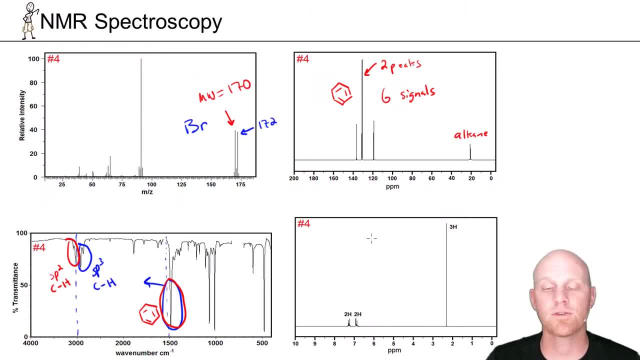 symmetry there. We've actually found out a fair amount of information before we've even gotten to the HNMR, but now we're going to spend the most amount of time in the HNMR. that's where the greatest amount of information is, So 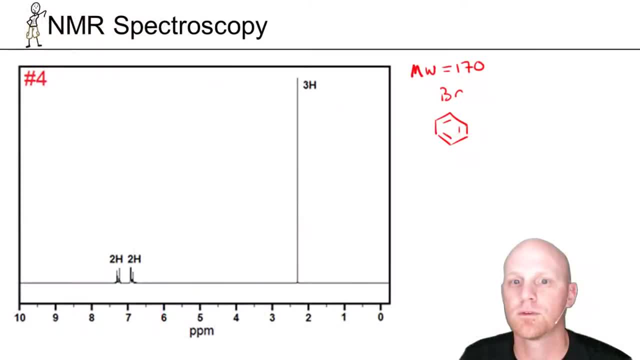 let's sort of look at that HNMR, So we'll definitely spend the most significant amount of time on our HNMR here. I highly recommend you get good at looking at your mass spec IR and carbon-13 NMR and just kind of breezing through them as 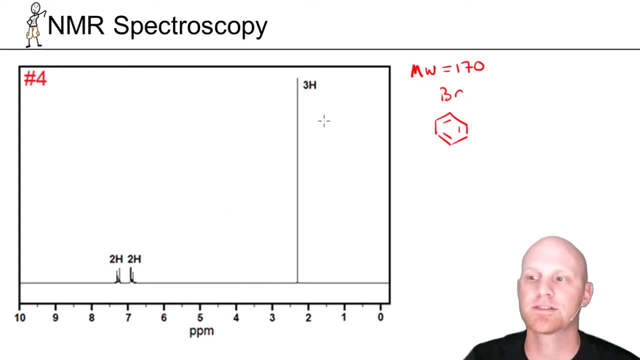 quickly as possible, because we're gonna spend the most time here In this case. I've just kind of diagrammed out that, yes, we already know the molecular weight is 170 and that there's a bromine from the mass spec and that we have a 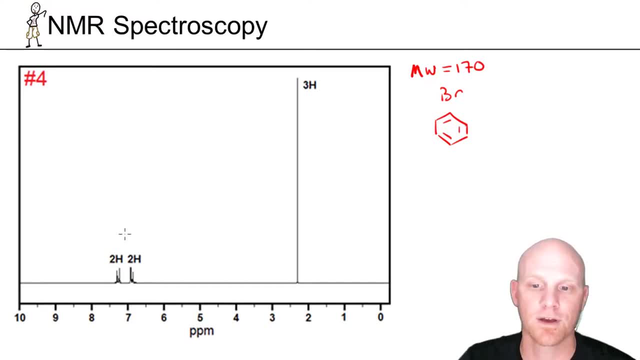 benzene ring both from the IR and the carbon-13 NMR and if we again still weren't sure, the HNMR here is going to confirm it In the aromatic region here between six and a half and eight and a half. we've got some signals, so we 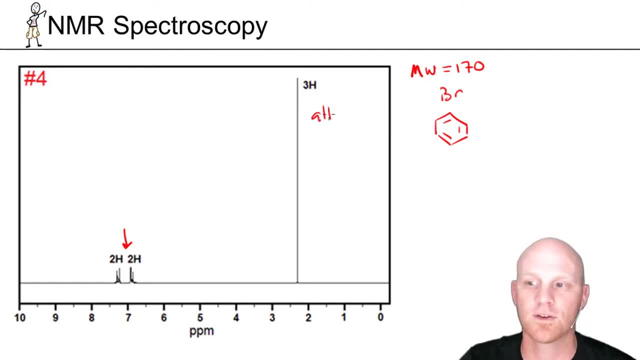 definitely have a benzene ring. We also have a one signal down here in the alkane region. Now in the alkane region I see this multiple of three and I like starting there, but it's the only place to start in the alkane region, since it's 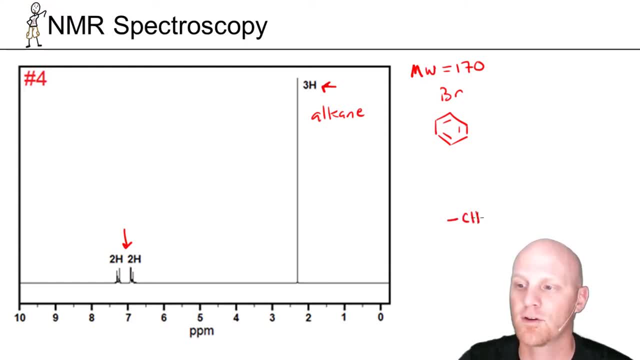 the only signal down there. But in that case that is a methyl group and I can see that it's a single peak, so a singlet, and so that tells me there's no neighbor. so I have no idea what this methyl group is next to at this point. It's just a. 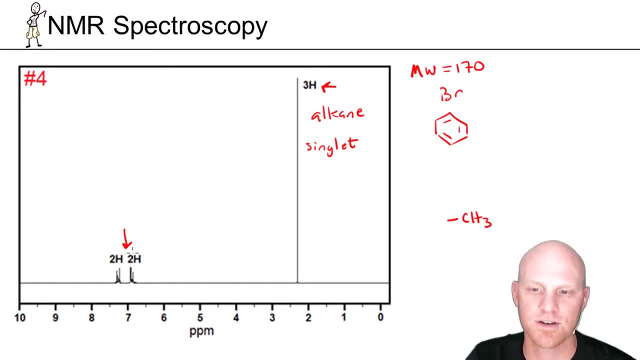 piece of the puzzle. So, and going back down to this aromatic region, we've seen this pattern before and I highly recommend it's one you commit to memory here. but we've got two doublets that it represents two H's each and that's a benzene ring with symmetry here, and we're gonna have two. 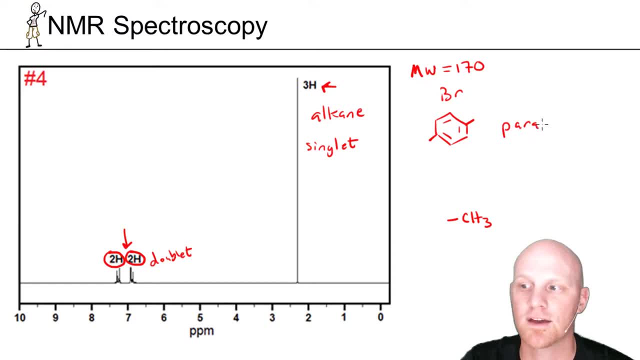 substituents coming off our benzene in a para disubstituted pattern on opposite sides. That way we maintain some sort of symmetry. And in this case we've interpreted all our signals. and the question we got to ask yourself is: do we have every piece of the puzzle? Well, in this case we don't know the formula, but 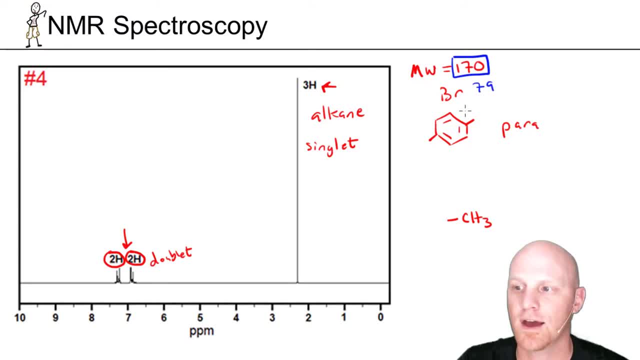 we do know it's going to weigh 170.. Well, bromine weighs 79. In this case, benzene ring with four hydrons on it, so six carbons is 72, plus the four H's gets us up to 76 and a methyl group is going to. 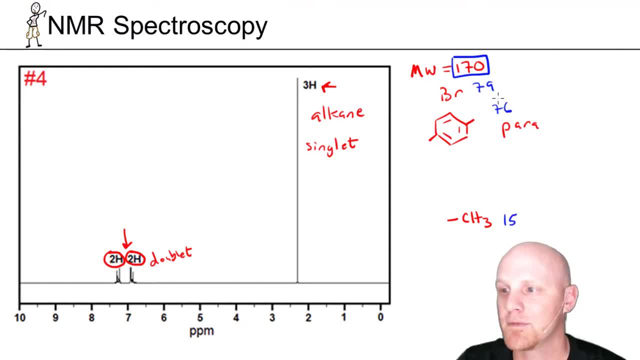 weigh 15, and if we add these all together here, in this case it actually does add up to 170.. So in this case, we do indeed have every piece of the puzzle, and the last thing that we need to do is just construct our molecule. So keep in.